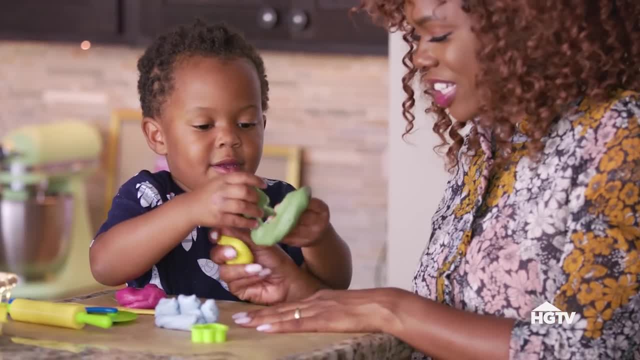 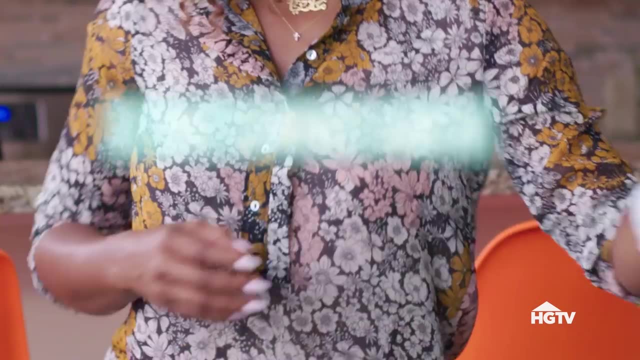 eat it, he's not gonna die. And two, it's super easy and fun to create, so let's get started. Here's what you're going to need for this project: Marshmallows, two teaspoons of coconut oil, three tablespoons of cornstarch and natural. 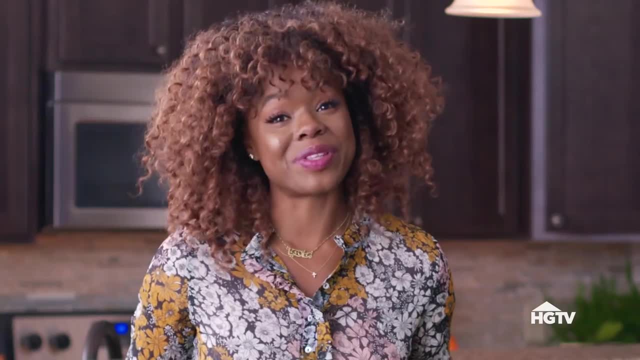 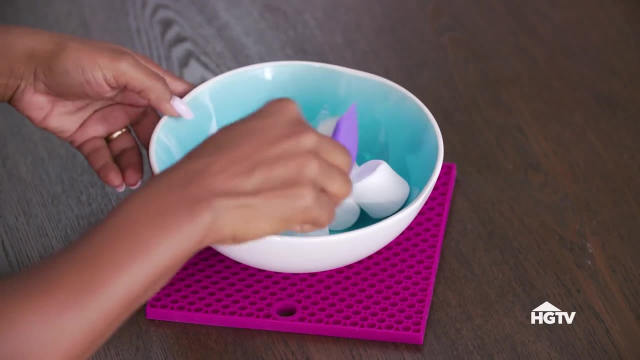 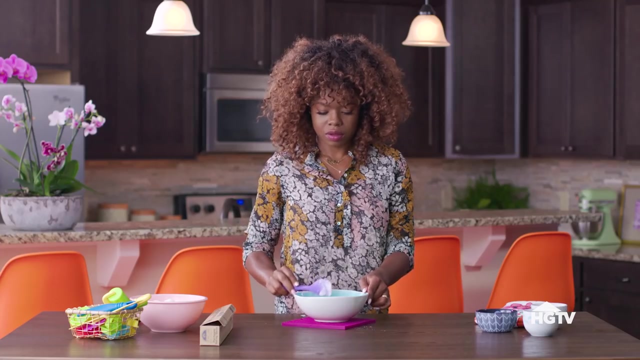 food coloring, because this is where all the creativity happens, Starting with six marshmallows in our microwave-safe bowl, two teaspoons of coconut oil. Next, we're going to take our three tablespoons of cornstarch, dump it in there, pour it into the bowl. Next we're going to take our food color. This is the fun. 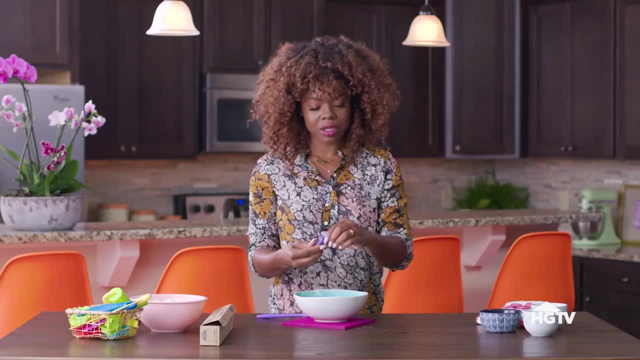 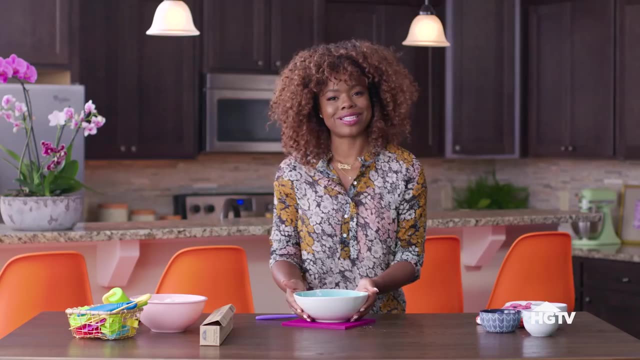 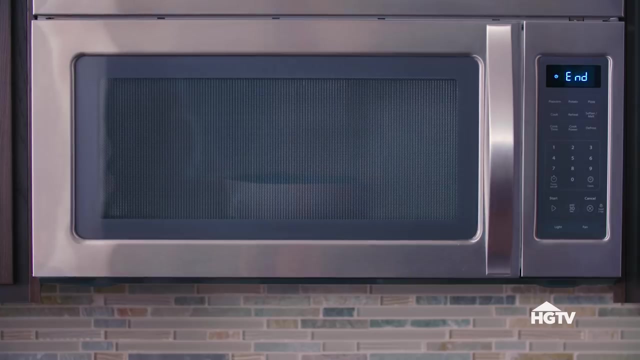 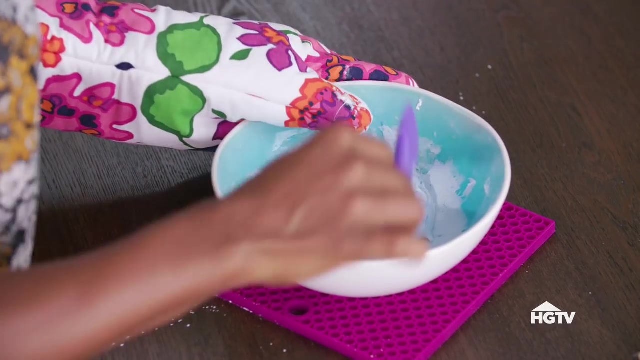 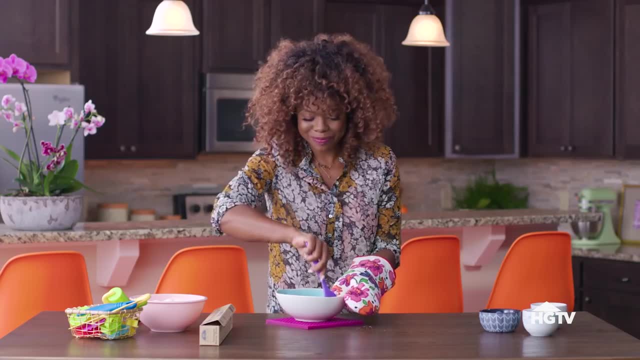 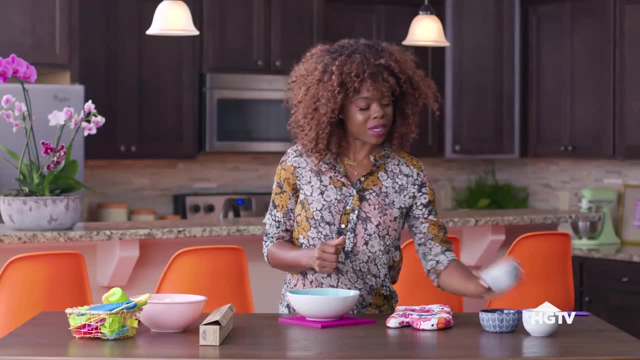 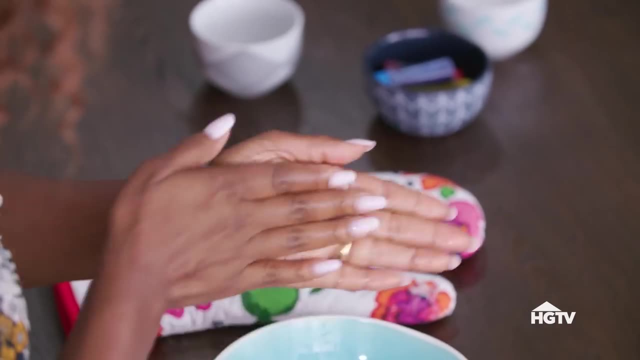 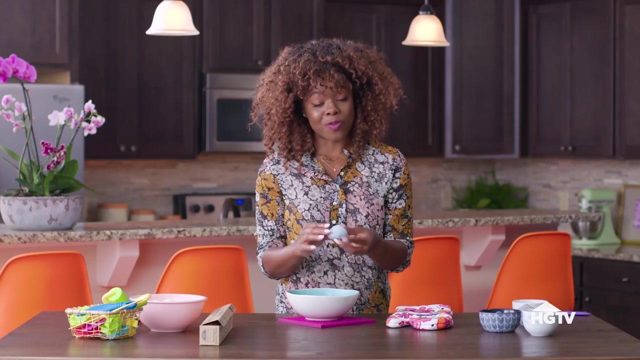 your marshmallow play-doh is cooled. you are now going to take remaining coconut oil. emulsify it in your hands. This is going to be like your barrier, so it doesn't get sticky. Pull it up and mold it With your marshmallow play-doh formed. 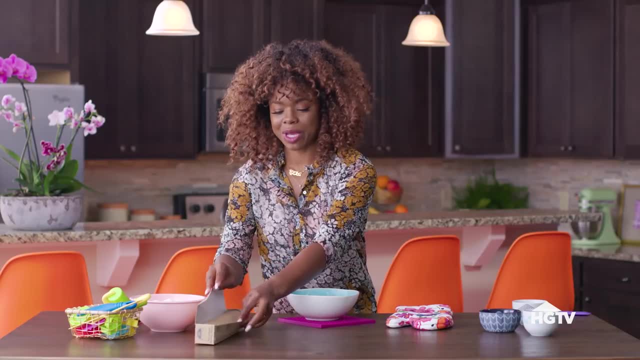 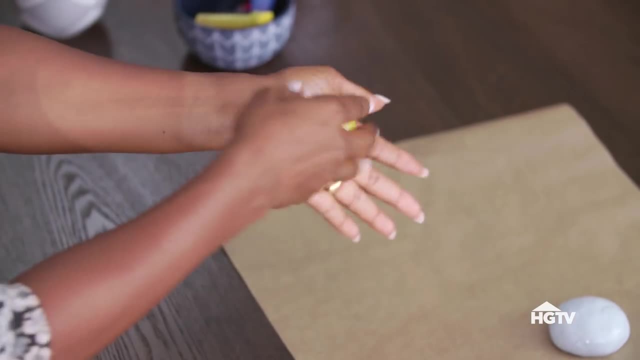 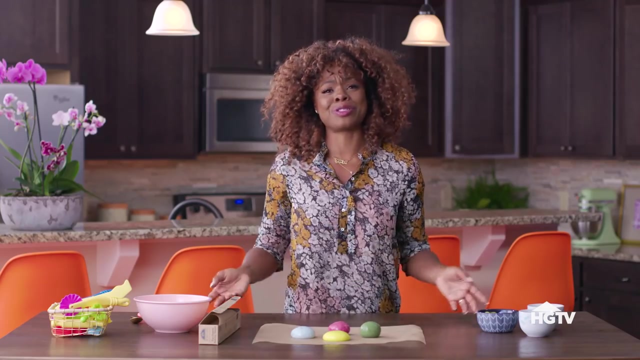 and ready to be played with. we're going to simply pull out a piece of parchment paper, Set it down. Now we just need a few more colors. Color options are endless. All you have to do is grab your kids and have a ton of. 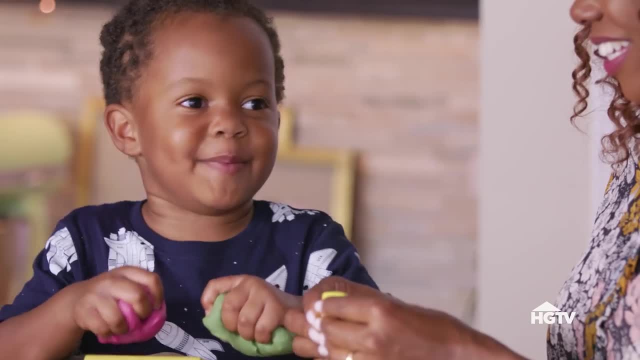 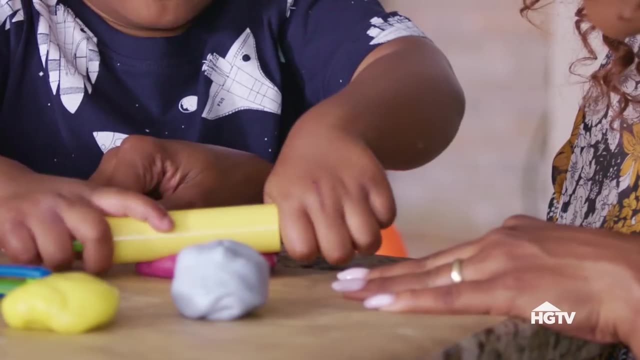 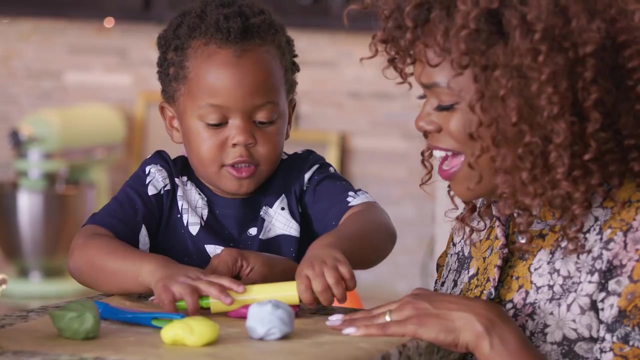 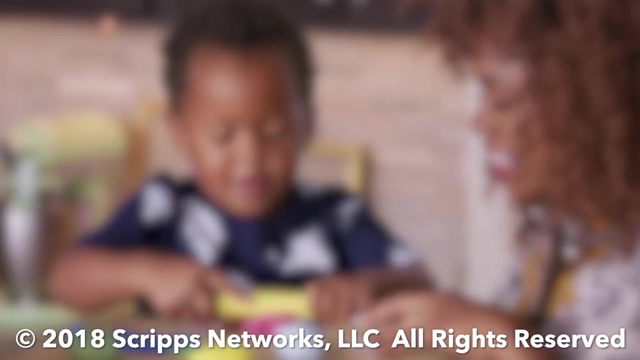 fun with your new marshmallow play-doh. It's marshmallow Yum. I hope this inspired you and I'll see you in the next one. you.